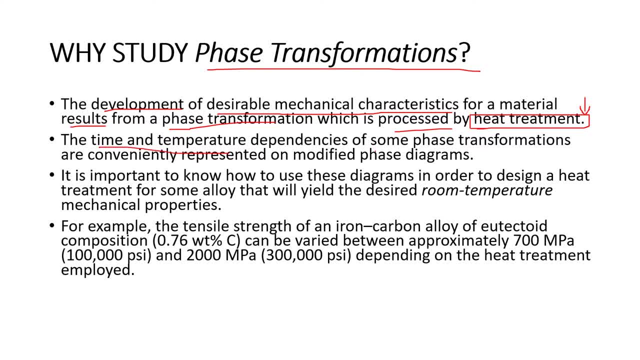 temperature potential of here heat field, which energy of beam, pressure of which effective result will be must be cure of heat. there is an evolution phase diagram also. we have already studied in the previous chapter or in this chapter, ten, which is an extension of the phase diagram. it is important to know how to use these. 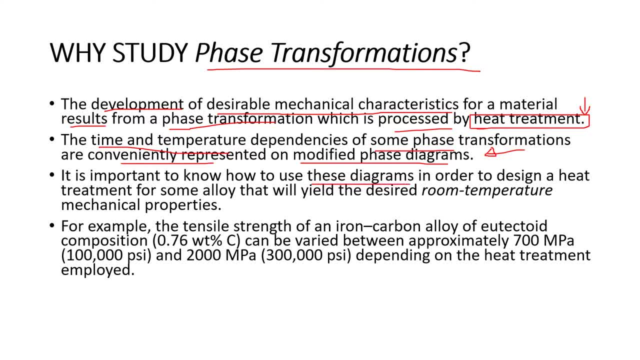 diagrams. we have already studied about how to read the phase diagrams in which different contact parts, fabrics, other things which can be't which related to basis of inchee, asked about to see what is built-in in the phase, to see how we can implement it when knees weighs an end that we will take you to the end barrell in a weather project. 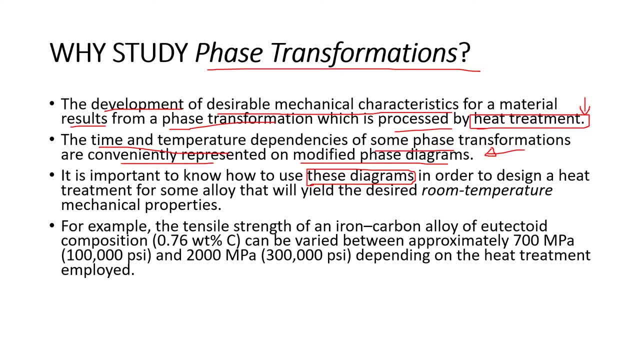 Compositions of a carbon or another ally was present and with respect to the change of temperature or pressure, We were studying the phase diagram. So, in order to design a heat treatment for some ally that will lead the desired room temperature, mechanical properties, for example the tensile strength of in. 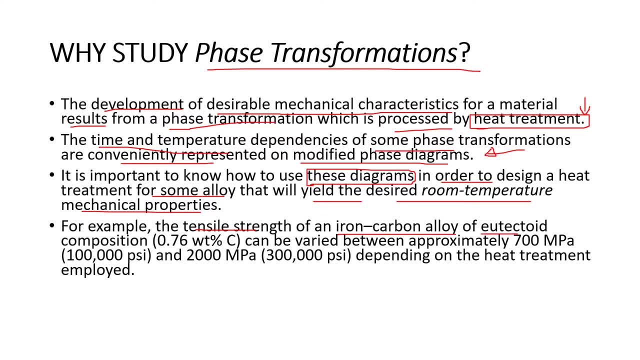 iron carbide, ally of a eutectide composition which is at zero point seven. six percent weight by carbon can be Improved or can be varied between approximately 700 megapascal, which is equivalent to hundred thousand psi, and 2000 megapascal, which is equivalent to three hundred thousand psi, which is much larger than the 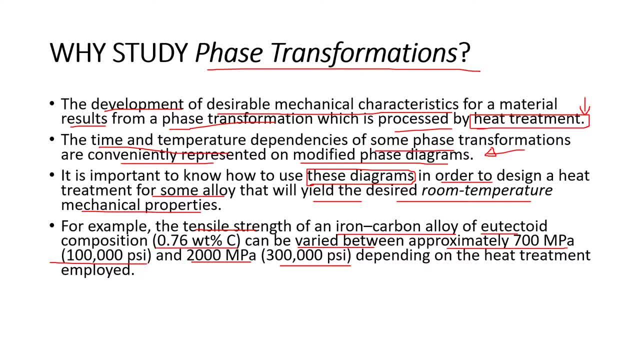 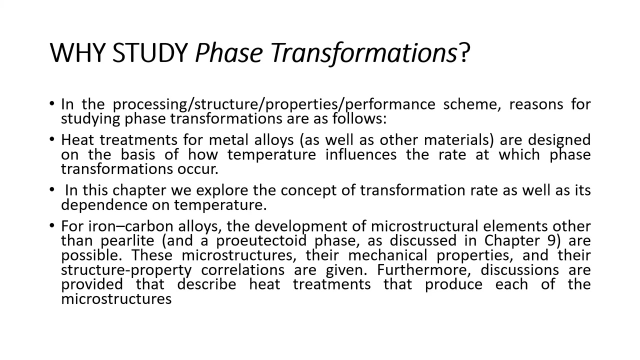 individual constituent, which is iron, if we combine it with an ally of carbon, So we can improve the mechanical properties From this range of 700 mega Pascal to 2000 mega Pascal, depending on the heat treatment used. Here we want to study Why, why we study. we want to explain why we study phases from transformation a bit more. 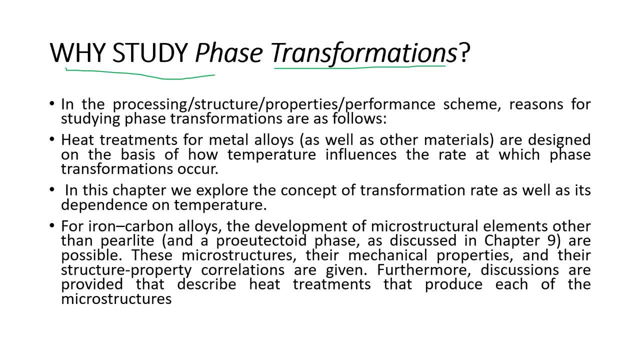 heat treatments of material, of metal allies as well as other materials, are designed on the basis of for how temperature influences the rate at which phase transformation occur. because, suppose it critical temperature, the phase transformation, it critical temperature must be different to then the phase transformation it above, at a temperature above the critical temperature range or 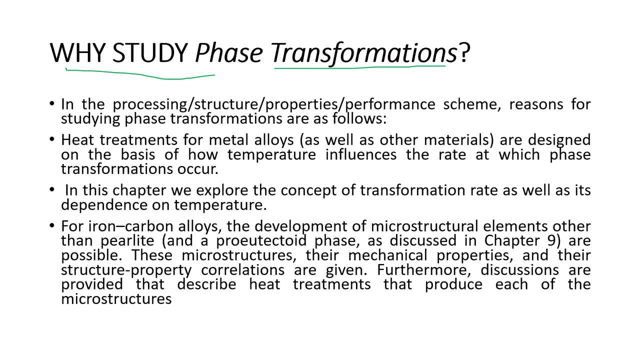 critical temperature. we call it eutectoid temperature for the iron-iron carbide diagram. if we study the example of eutectoid reaction, we can know how the heat treatment of metal, how it influences, how the temperature influences the rate at which phase transformation occur. 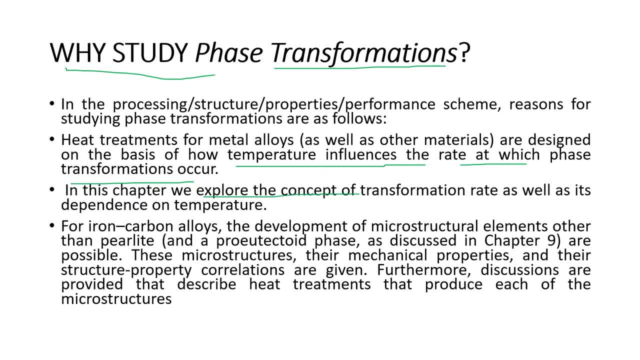 So in this structure we further explore the concept of transformation rate. Transformation rate which will depend upon the temperature, as well as the formation, the formation, the types of formation and the mechanism of the formation, the kinetics of phase transformation. we will study these effect. 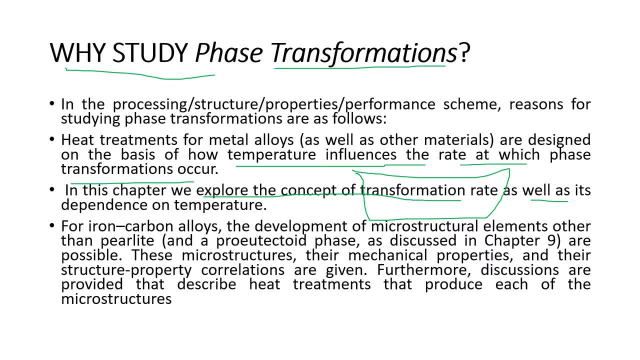 So for iron-iron carbide alloys, the development of the microstructure elements other than pearlite and pro-eutectite phase is we have discussed in chapter 9, or possible, Like one other example, For chromium nickel-chromium alloy. we have already discussed in chapter 9 about nickel-chromium. 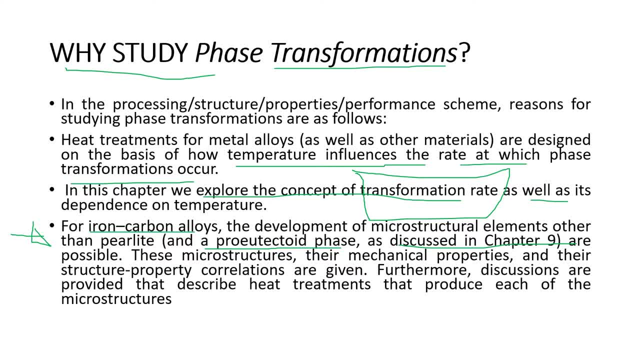 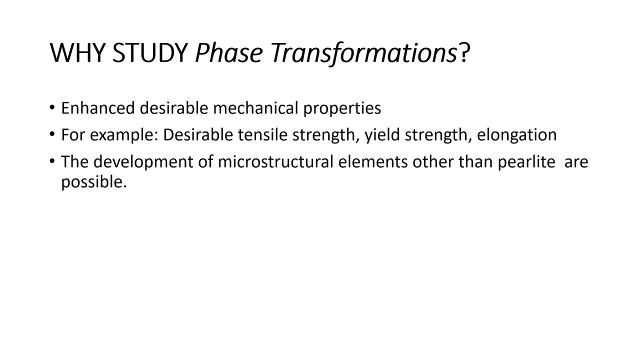 alloy is other than iron-carbide alloy. So these microstructures, their mechanical properties and their structural property correlations are given. Furthermore, discussions are provided that describe heat treatments that will that produce each of the microstructures. Why we study phase transformation. 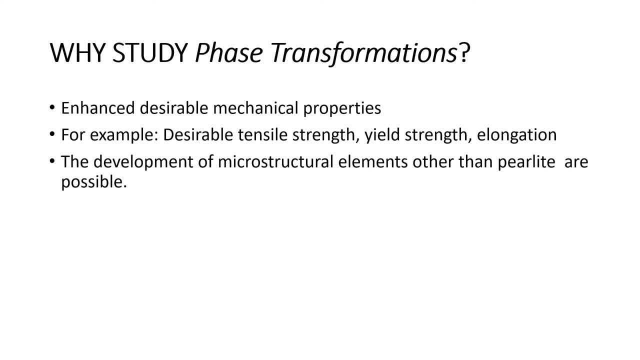 We study phase transformation in order to enhance the desirable mechanical properties. This is the summary Why we study. We want to improve the mechanical properties of the structures, For example, desirable tensile strength, Yield strength And the resistance And elongation. 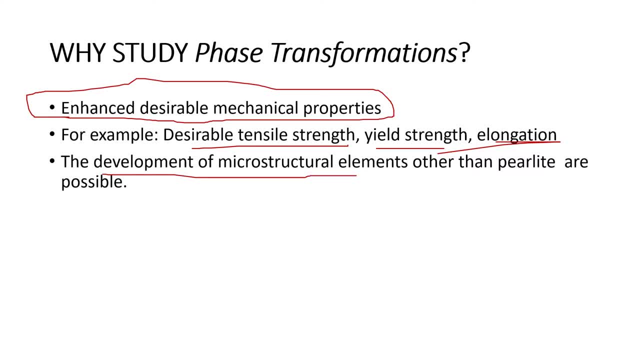 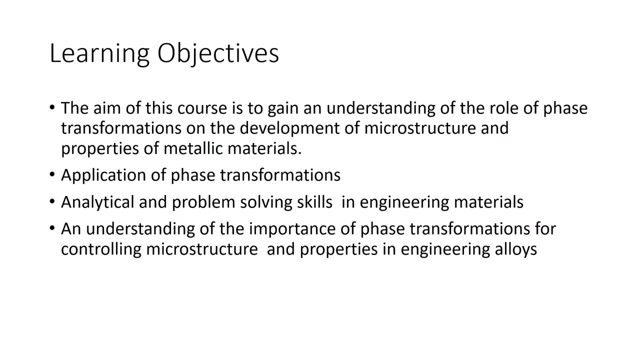 The development of microstructure elements other than pearlite are possible. For example, we have studied the phase diagram of nickel-chromium alloy. Our learning objectives: we have already discussed our learning objectives in the phase transfer while in the previous slide, But let's summarize our learning objectives in this. 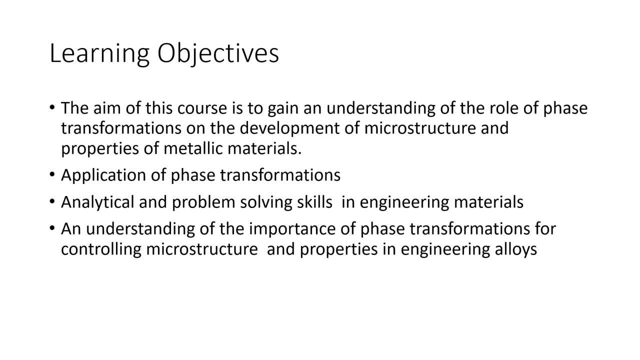 in this lecture in the last two lecture lecture the learning objectives of the chapter lecture number 29 and 28 and 30th is. the aim of this course, of which is related to phase transformation, is to gain in understanding of the role of phase transformations on the development of microstructure and properties of. 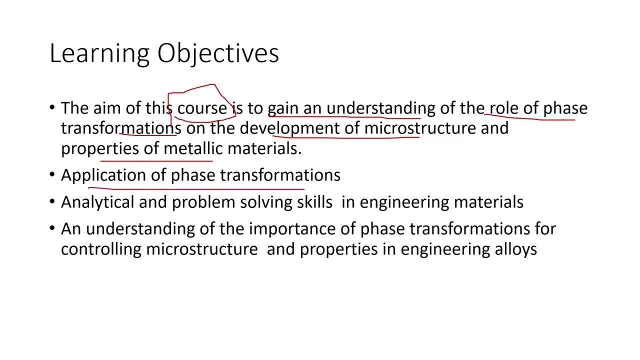 metallic materials. applications of the phase transformations, analytical and problem-solving skills in engineering materials. we will study some examples, some solid examples from the book of Sylvester, regarding the nucleation formation, regarding the growth formation which affect the phase transformation, an understanding of the importance of phase transformations for controlling 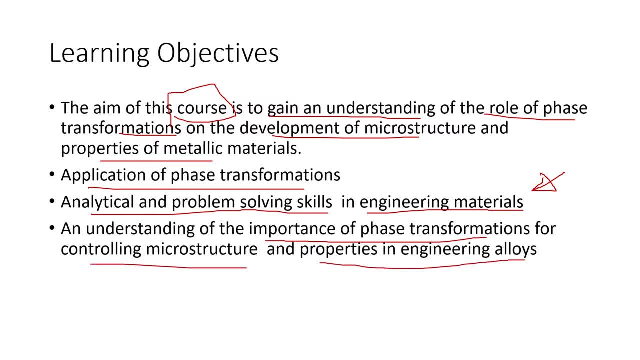 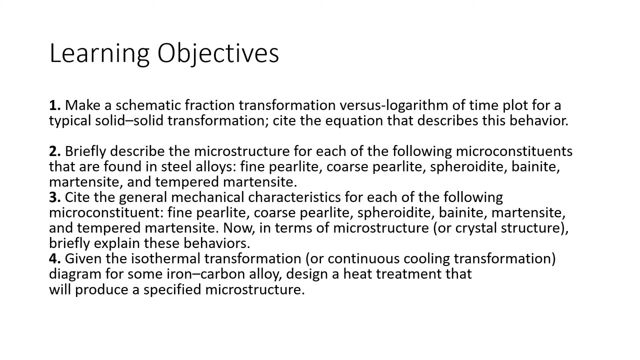 microstructures and the properties in engineering allies. we will solve some equations, some numerical equations which we will simulate in MATLAB to plot the curves in order to study the effect of the nucleation formation and growth rate, make another the summary of the learning objectives or make a schematic fraction transformation. 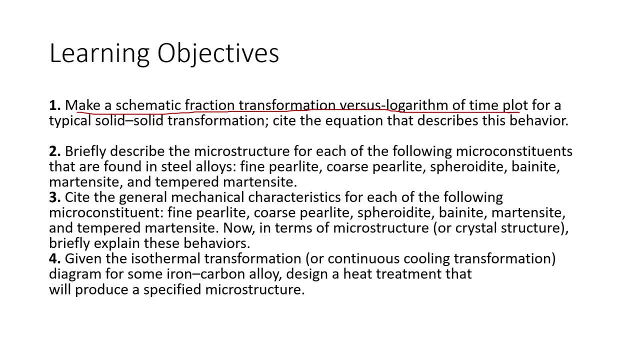 versus a logarithmic of time plot for a typical solid, solid transformation side. the equation that describes this behavior. we will study the in some equations for the description of the behavior of the kinetic formation. briefly describe the microstructure for each of the following micro structures that create crazy: 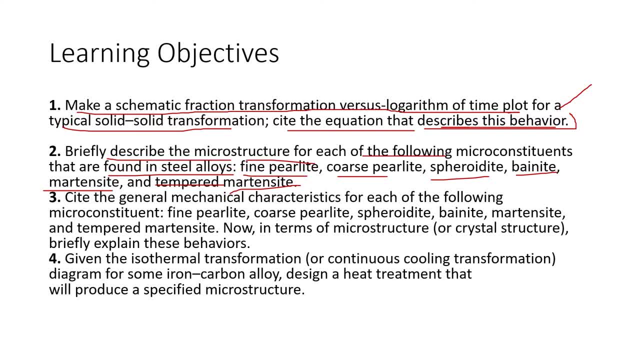 constituents that are formed in steel alloys, like fine pearlite, horse pearlite, spheridigm, benetite, martensite and temperature denput martensite. number third one is cite the general mechanical characteristics of each of the following micro constituents: fine pearlite, coarse pearlite, spheroidite, ventite martensite, tempered martensite. 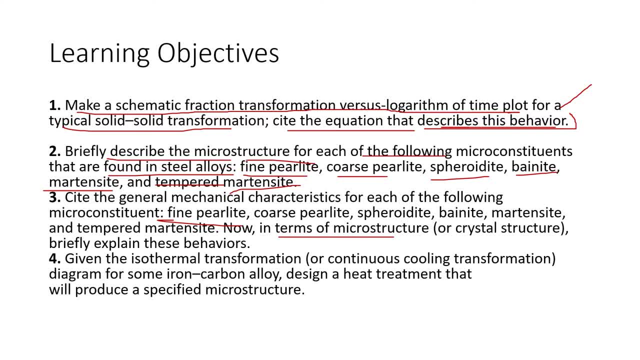 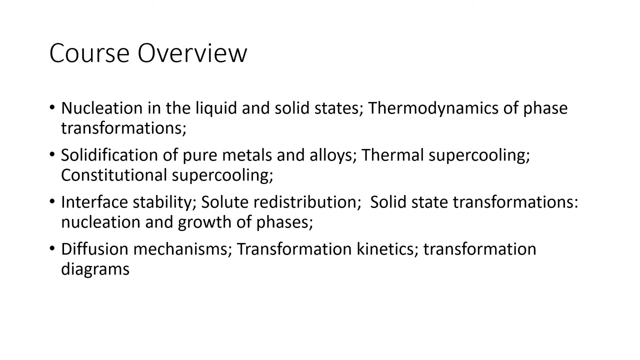 Now, in terms of microstructure or crystal structure, briefly explain these behaviors. Given the isothermal transformation or continuous cooling transformation diagram for some iron-carbon alloy design, a heat treatment that will produce a specified microstructure. The course overview is the nucleation in the liquid and solid states. 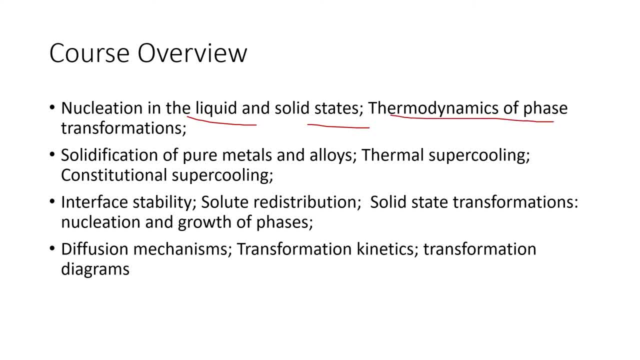 thermodynamics of phase transformations, solidification of phase transformations. solidification of phase transformations for pure metals and alloys, thermal supercooling, constitutional supercooling, interface stability, solute redistribution, solid states, transformation, nucleation and growth of phases. 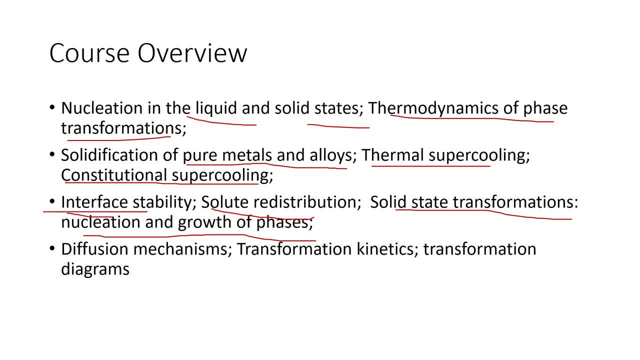 These topics. the nucleation: I will focus mostly in this chapter about the nucleation and growth formation. this is the main part of this chapter: nuclear nucleation and growth formation, growth of phases, diffusion of mechanics, transformation, kinetics, transformation diagrams. however, thermodynamics of phase transformation, i will not study this. 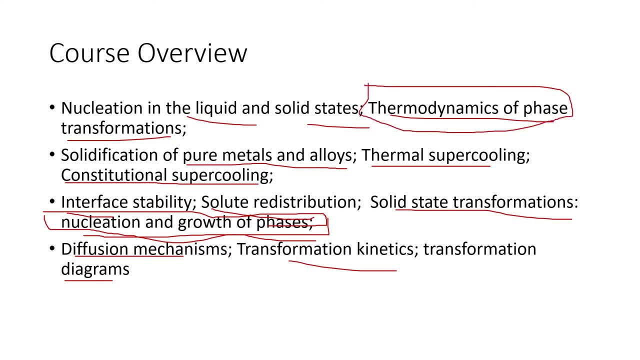 in detail because i will deviate from the main: phase transformation, although thermodynamics of phase transformation is one of the part of the formation of nucleation, but we will study some basic principles of the thermodynamics of phase transformations like entropy and enthalpy. these are the some basic concepts of the nucleation formation. 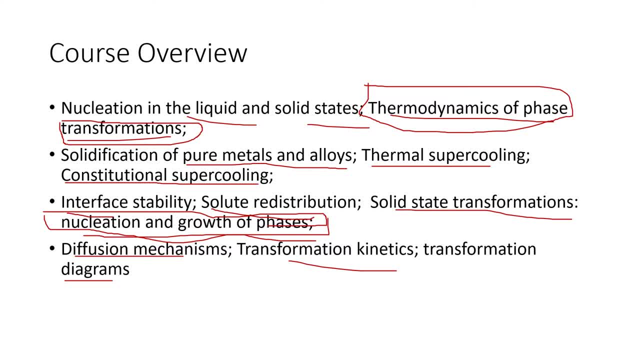 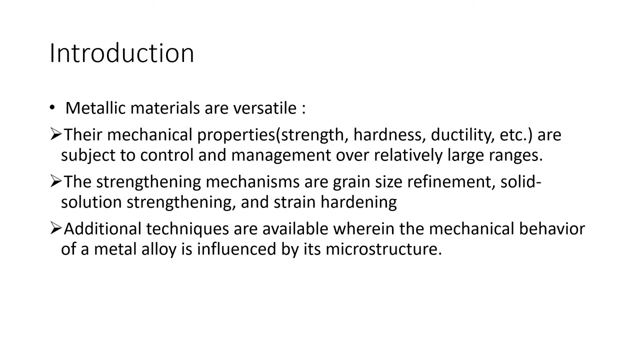 we will study only the effects of the thermodynamics. the thermodynamics, we will study only the thermodynamics effects of the phase transformation. but mainly we will discuss the nucleation form and growth formation in solid states in thermal super cooling and constitution super cooling. introduction: metallic materials are versatile. 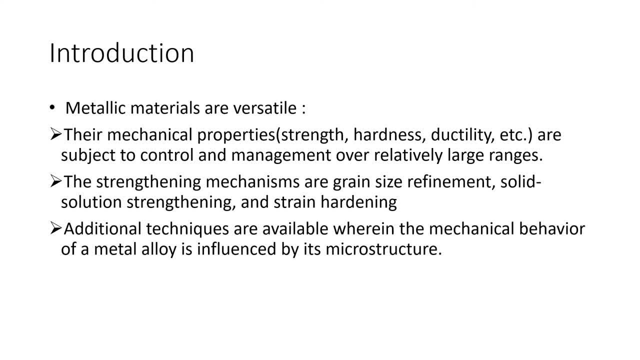 their mechanical properties- strength, ductility, hardness- are subject to control and management over relatively large ranges. so these strengthening mechanisms are already discussed by mr Mohsen in the previous lectures. these strengthening mechanisms are namely: grain size refinement, solid solution strengthening, strain hardening. some additional techniques are available, like mechanical behavior of metal alloy influenced by the micro structure. 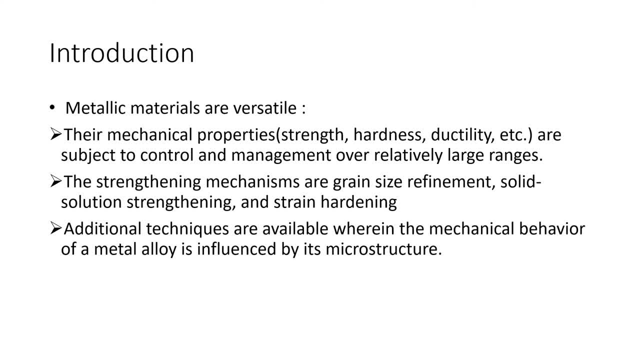 like i have discussed in the phase diagrams and i have also discussed in the phase diagrams, the development of micro structure in both single and two phase ally ordinarily involves some type of phase transformation in alteration, the additional like alteration in the number or characteristics of the phases. the development of micro structure involves the single and two phase. 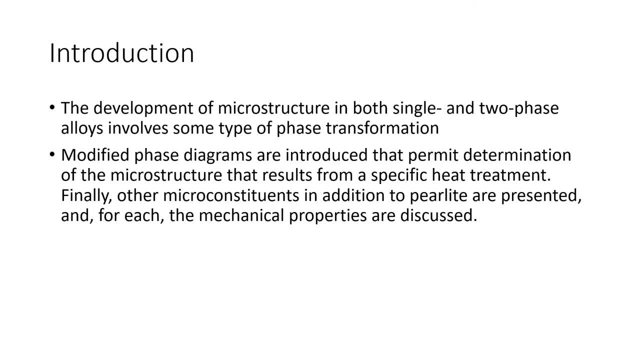 alteration in the number or characteristics of the phases. The development of both of microstructure in both single and two phase alloys involves some types of phase transformation. So modified phase diagrams are introduced that permit determination of the microstructure that results from the specific heat treatment. 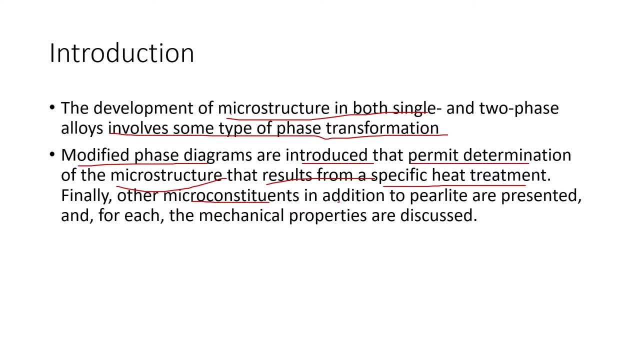 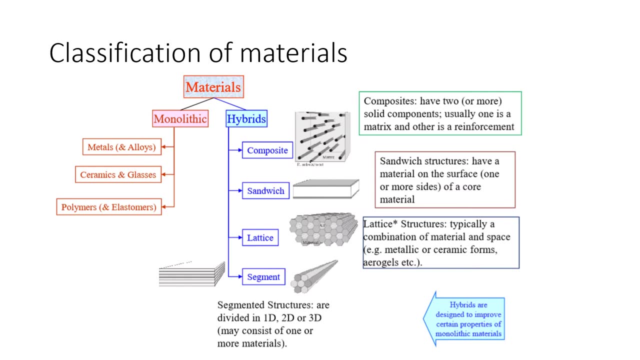 Finally, other microstructurants in addition to pearlite are presented, and for each the mechanical properties are discussed. in this lecture Phase, transformation is very important, So we want to focus on some specific topics, But before this we want to classify some materials. 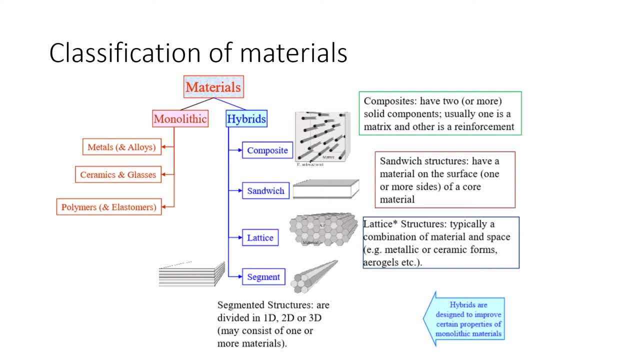 So we want to classify some materials, But before this we want to classify some materials For the phase transformation. that's why in the classification of the materials the materials are divided into two main types, So one is monolithic, the other is hybrid. 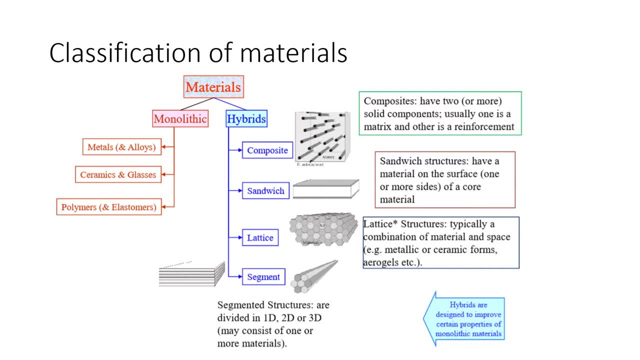 Further monolithic materials are further divided into some parts, like metal and alloys, ceramic and glasses. Further monolithic materials are further divided into some parts, like metal and alloys, ceramic and glasses, Polymers and elastomers. The other part is hybrid. 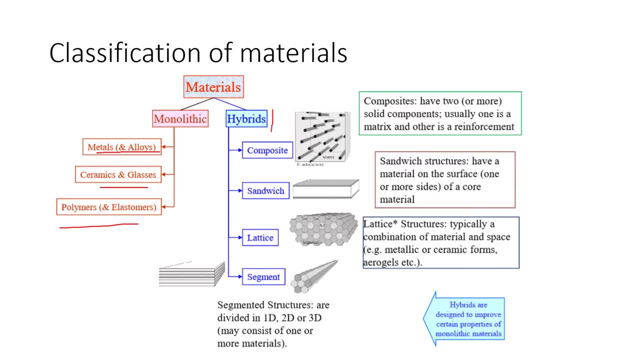 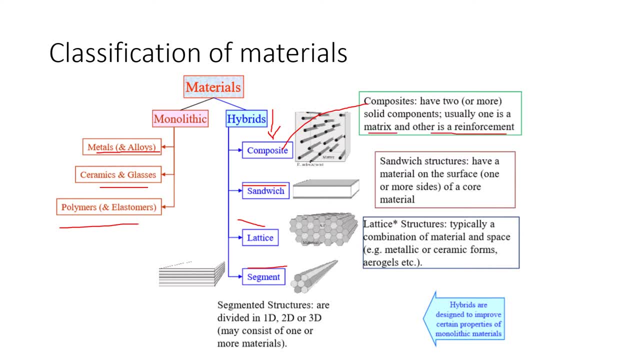 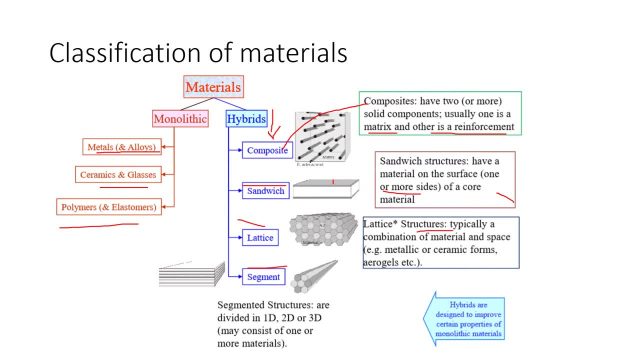 Latest structures, typically a combination of material and space, For example metallic or ceramic forms. For example, metallic or ceramic forms. Segment structures are divided into 1D, 2D, 3D may consist of more materials. Segment structures are divided into 1D, 2D, 3D may consist of more materials. 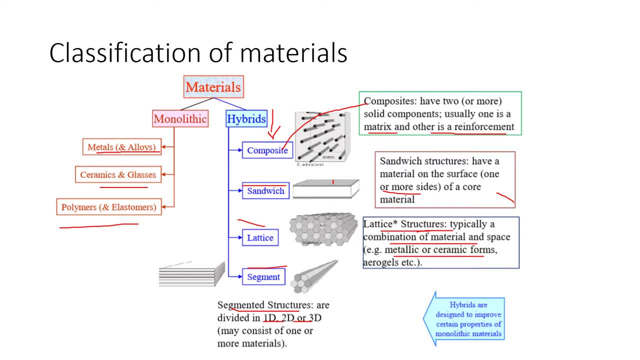 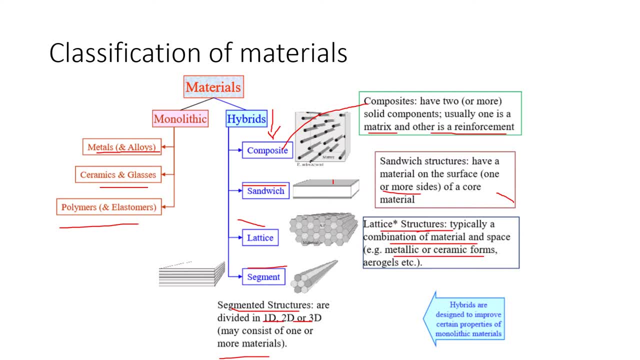 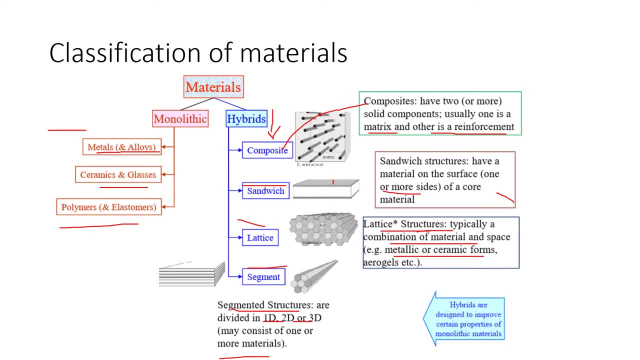 Hybrids are designed to improve certain properties of monolithic materials. These are the monolithic materials. These are the monolithic materials. Hybrids are designed to improve certain properties of monolithic materials. Hybrids are designed to improve certain properties of monolithic materials. 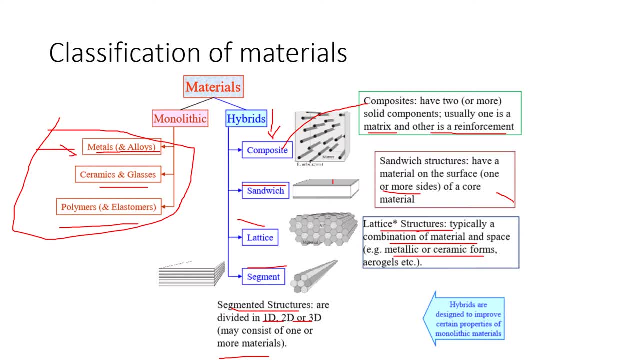 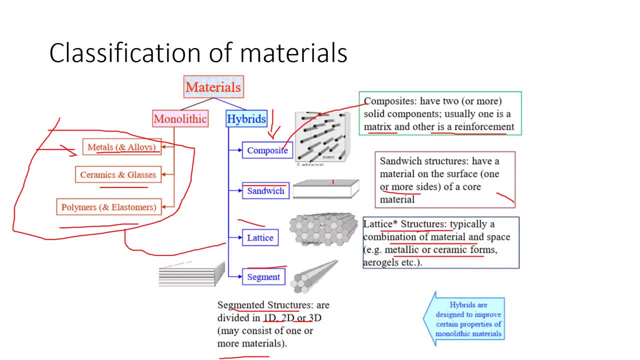 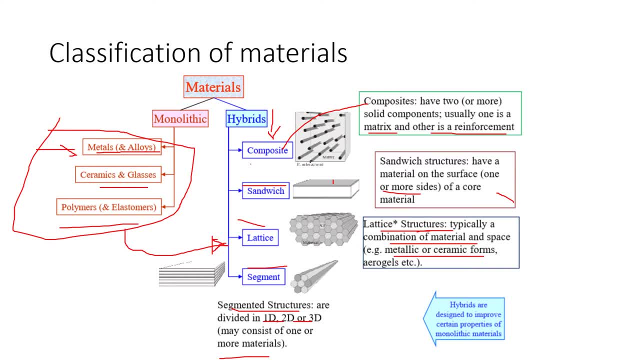 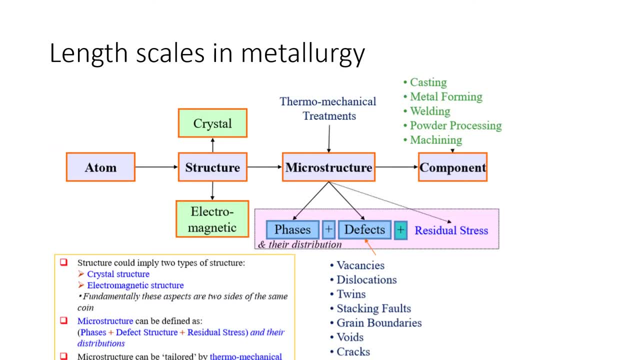 Length scales in metallurgy. Basically, all the universe is form of the atom And every time, all the time we see about the structure, Structures are formed by the crystal forms and electromagnetic form. Similarly, microstructures. if we study the behavior of the structure, we see that the structure is formed by the crystal forms and electromagnetic form. 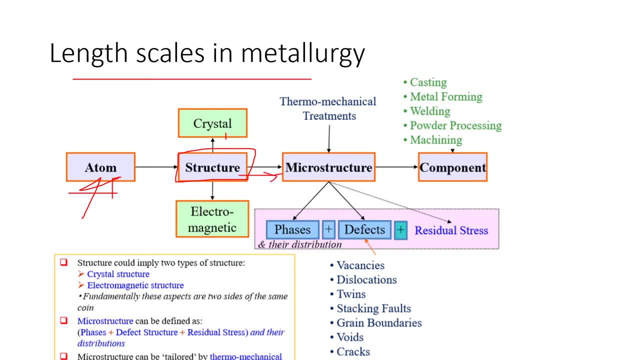 Similarly, in the case of the structure, we go to the microstructures. In the microstructures, we study the thermomechanical treatments In order to improve- we want to improve the properties of the structure. The structure is formed from the crystals or electromagnetic material, electromagnetic properties, 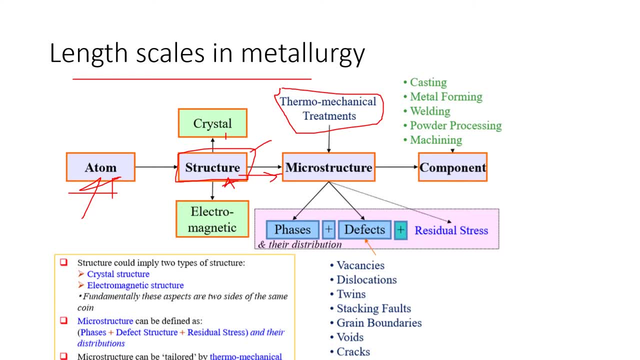 In order to improve the properties of the structure, we go to the microstructure. We further study the microstructure. We study the microstructure behavior. In the microstructure behavior there are thermomechanical treatments like heat treatments and phases, And we study the defects. 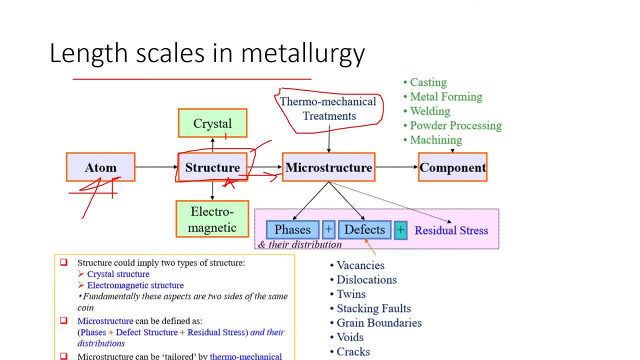 While we study the microstructure behavior of material, we study the phase transformation. We study the phases, different phases, single phase, two-phase alloy system or multi-phase alloy system. We study the defects. We also study the residual stresses. We relieve these residual stresses through heat treatment processes. 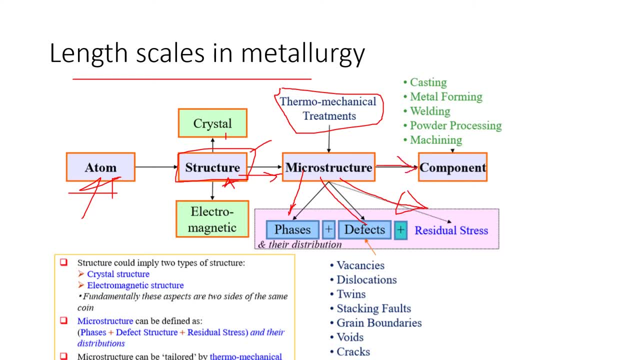 For this we can get the component, the main constituent, The components are formed. the formation of the component, which is formed from the several procedures like casting metal forming, Welding powder, processing or machining, Structure code implies into two types of structure: crystal structure and electromagnetic structure. 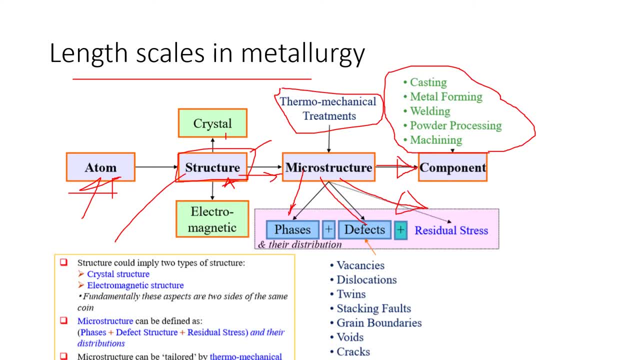 Microstructure can be defined as phase defect structure, residual stresses And the defects In the phases. we usually study binary phase Or single phase. And what could be the possible defects: Vacancies, dislocations, twins, stacking faults, grain bodies, voids, cracks. 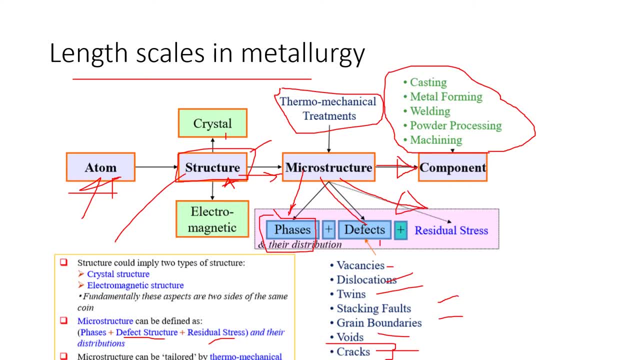 Based on the cracks. we study the material failure analysis. We study the cracks, We study the microstructure behavior And the microstructure behavior. We study about the voids, grain bodies and craters. We can calculate the life of that structure. 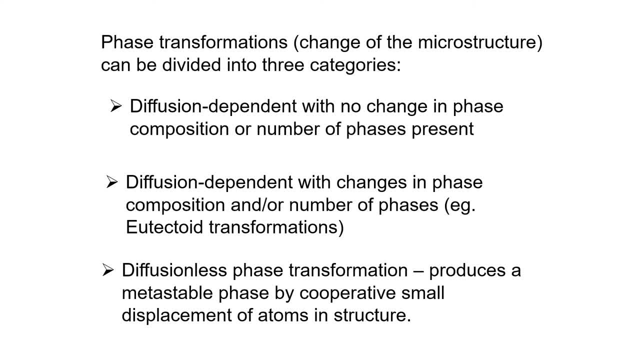 Phase transformations is actually the change of the microstructure. This can be divided into the process can be divided into three categories: Diffusion dependent with no change in phase composition Or number of phases present. Diffusion: the second type is diffusion dependent with changes in phase composition. 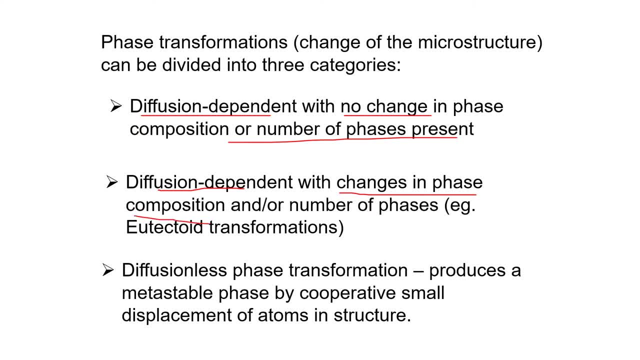 The first one is the diffusion dependent with the no change in phase. The second one is diffusion dependent with changes in phase compositions Or number of phases, For example, eutectoid transformation. If you can't believe or if you want to go to the details of the changes in phase composition, 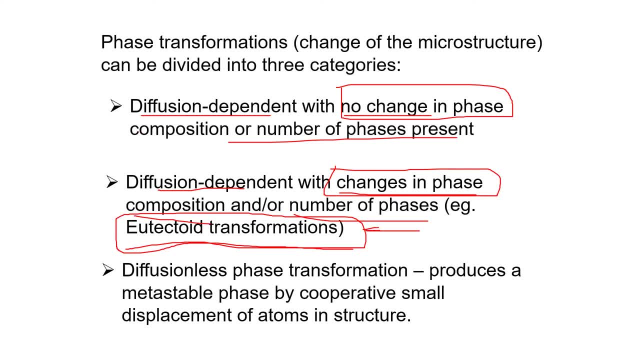 Go to the eutectoid reaction which we have already studied In iron-iron carbide diagram. The third type is: the first one is diffusion dependent. The first two parts are diffusion dependent. These two parts are diffusion dependent with no change and with change in phase transformation. 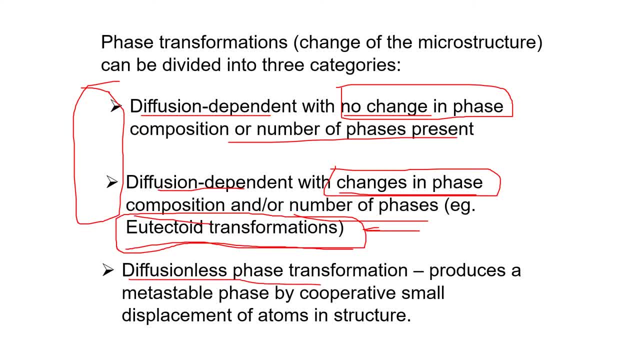 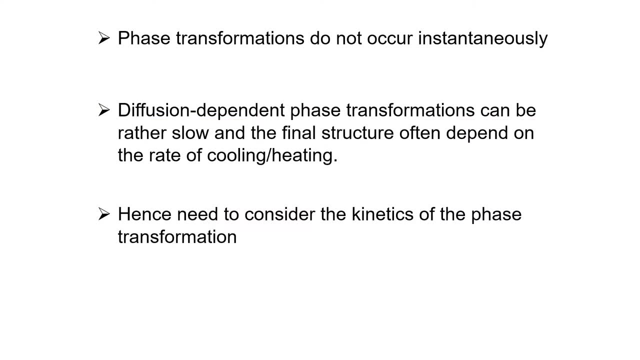 The third one is diffusionless phase transformation. This produces a metastable phase by cooperative, small displacement of atoms in the structure. Phase transformation do not occur instantaneously, which we have already studied. in this behavior They do not occur. the phase transformation do not occur instantaneously. 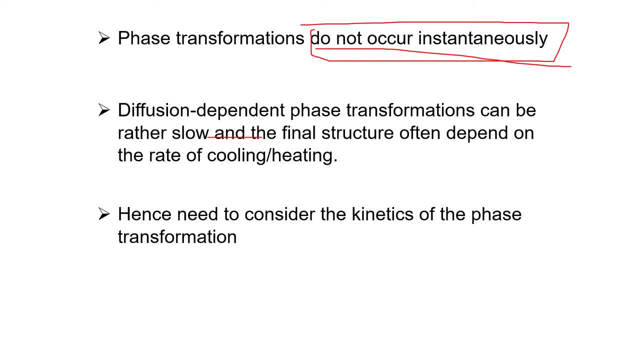 Diffusion dependent phase transformation can be rather slow And final structure often depend on the rate of cooling or rate of heating Which is a part of the heat treatment process. So diffusion dependent process depend upon the very slow cooling or very slow heating. The final structure depends upon the very slow rate of cooling or heating. 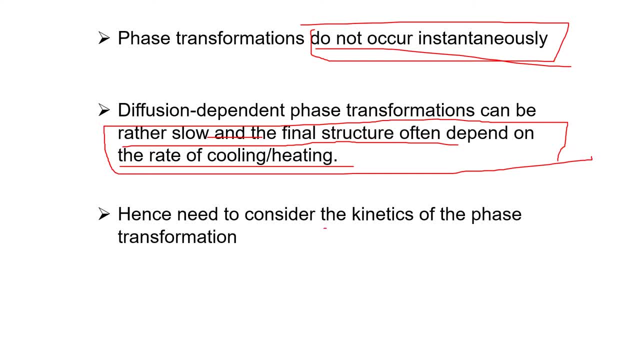 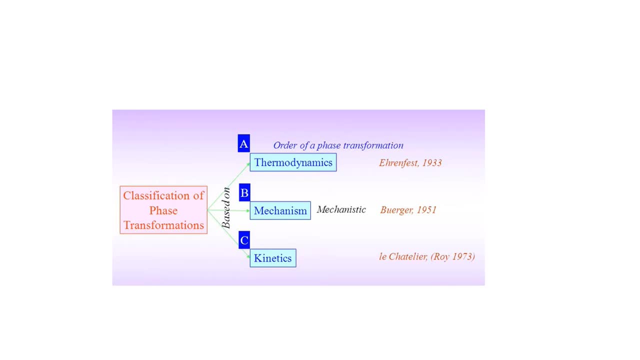 Hence need to consider the kinetics of the phase transformation. So we will study the kinetics of phase transformation For this purpose. The order of classification of phase transformation can be further divided into three types. One is the- A is thermodynamics, Which depends upon the, which is which was basically studied by this scientist in 1933.. 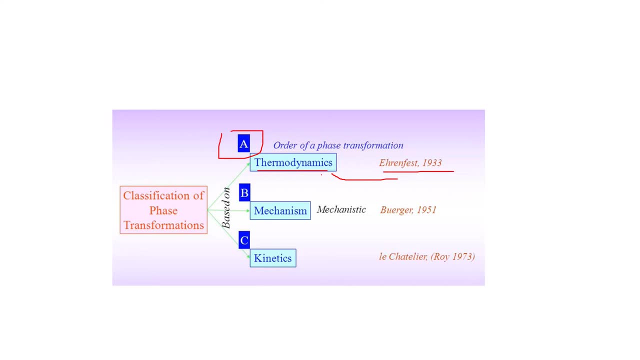 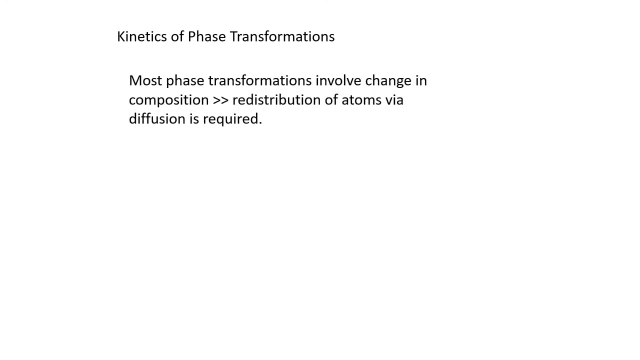 So this is the first type, And the other classification is based on the mechanism. The third one, it is based on the kinetics- Kinetics of phase transformation. Most phase transformation involve change in the composition. Like, for one, is the most common example of iron-iron carbide diagram: 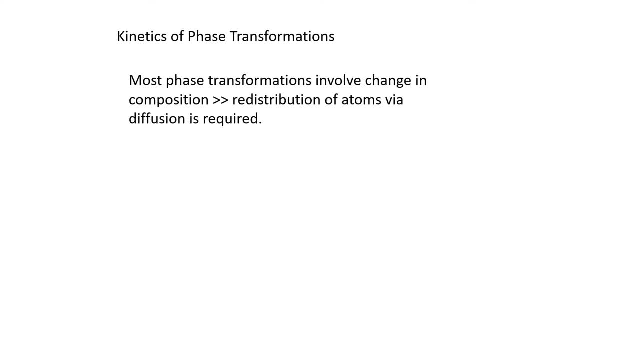 In which the carbon composition is changed. Redistribution of atoms where diffusion is required. This process involves nucleation of new phase, Formation of stable small particles. Nuclei of new phase Nuclei are often formed at grain boundaries and other defects. 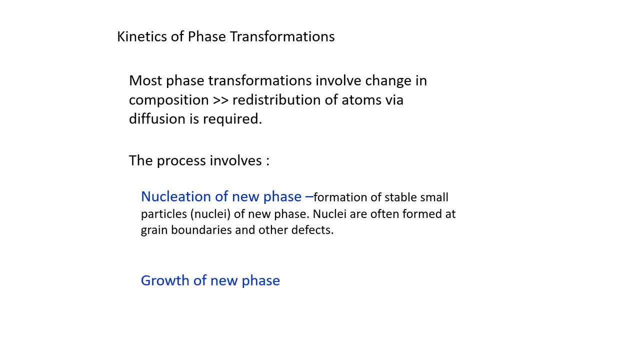 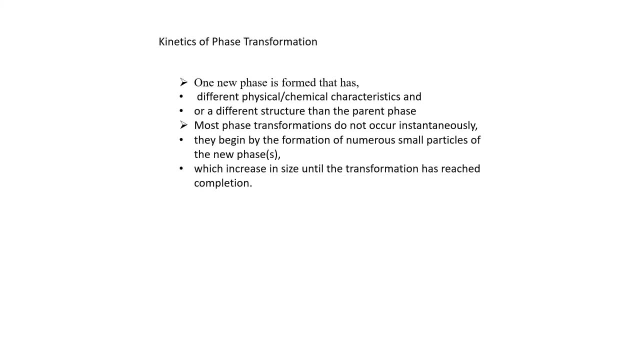 Growth of new phase. Kinetics of phase transformation. With the phase transformation, normally At least one new phase is formed That has different physical or chemical characteristics Or different structure than the parent phase. So one new phase is formed that has different physical or chemical characteristics. 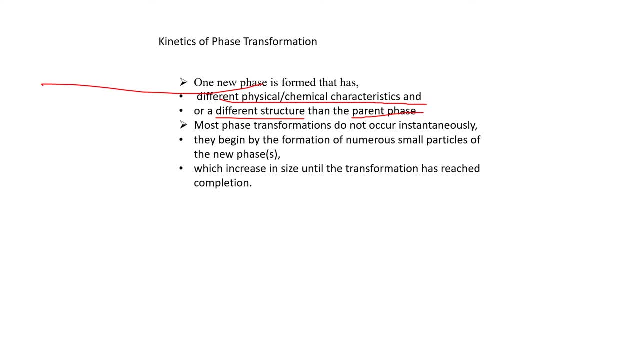 Or different structure than the parent phase. For example, most of the time we are discussing chromium nickel properties. Chromium nickel properties are the chromium properties. The parent phase is chromium, While new phase is formed in the form of chromium nickel alloy. So most of the phase transformations do not occur instantaneously. 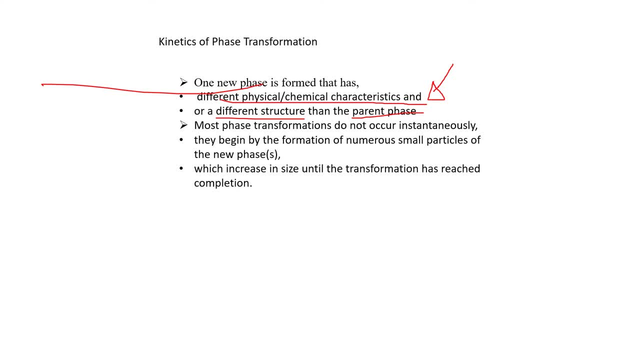 Rather, they begin by the formation of numerous small particles of the new phases, Which increase in size until transformation has reached completion. This transformation depends upon, by increasing either the temperature or the pressure of the alloy, Or the composition, or the change of the composition. 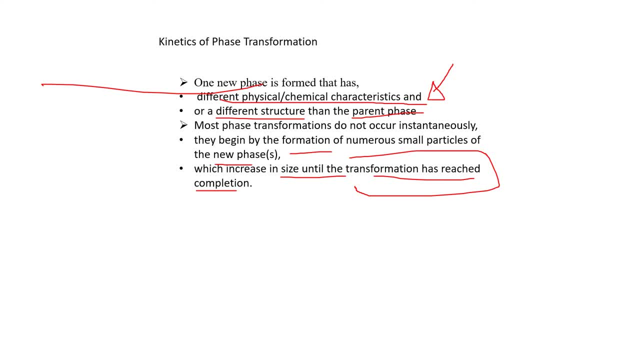 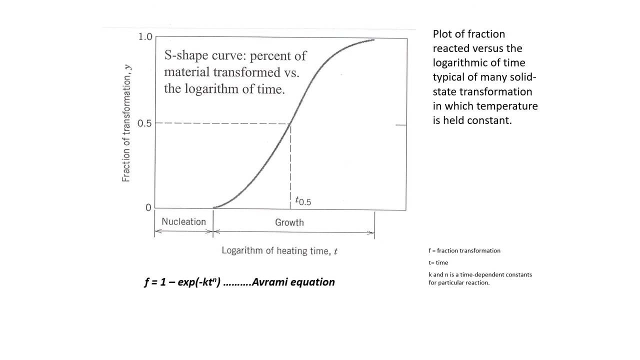 So the small particles begins, Numerous small particles begins, Which increases the size Until the transformation has reached completion. The progress of phase transformation may be broken down into two distinct stages. One is the nucleation, The other is the growth. So this graph explains the formation of small particles begins to form until the formation is complete. 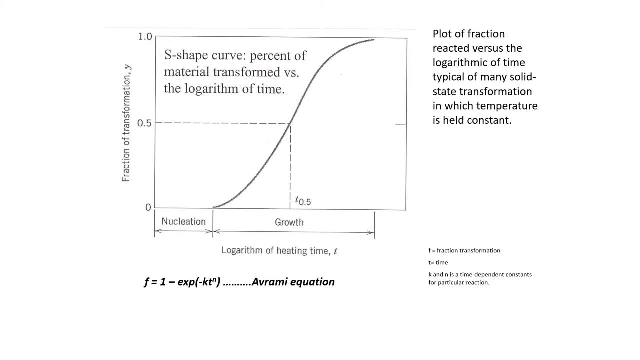 The nucleation, The range of the nucleation, The two range, Because the progress of phase transformation broken down into two types: One is the nucleation, The other is the growth. The range of the nucleation. In this plot, the range of the nucleation and growth is given. 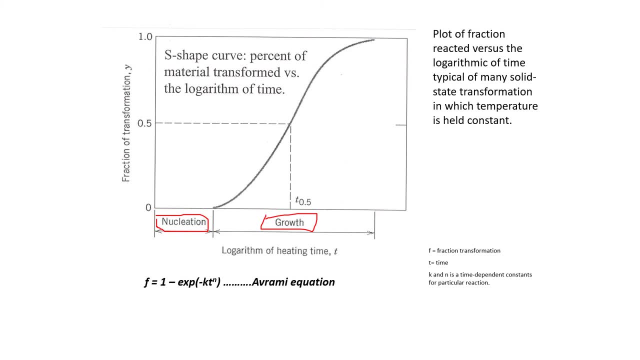 Nucleation involves the appearance of form. Very small particles are nuclei of the new phase, Often consisting of only few hundred atoms Which are capable of growing Like suppose. first nucleation forms From few forms in the horizontal line And in the horizontal axis. 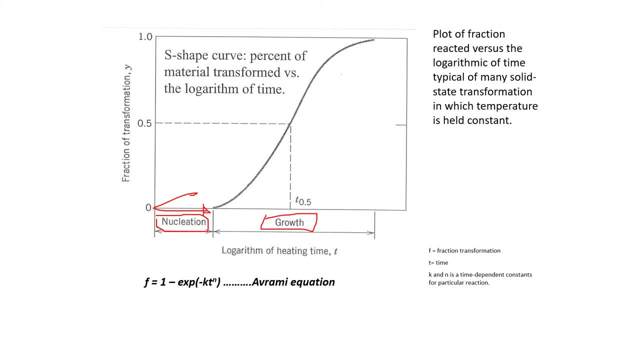 Nucleation. Initially the nucleation begins Over here, From the small particles. The nucleation involves the appearance of. Over here, in this range, The appearance of very small atoms begins to form Few hundred of atoms. It ranges After the nucleation. the growth starts. 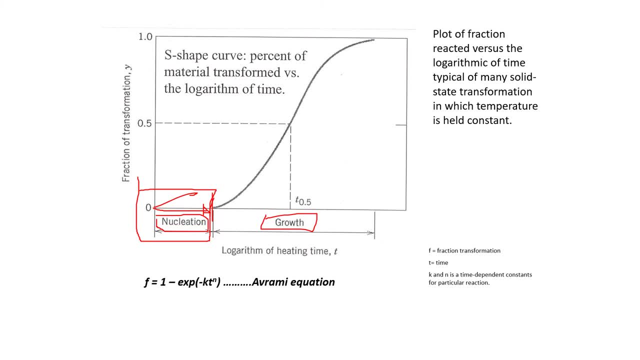 During the growth stage, These nuclei increase in size. The vertical axis Fraction of transformation Is mentioned from range Between zero to one. During the growth stage, These nuclei increase in size, Which results in the disappearance of some Or all of the parent phase. 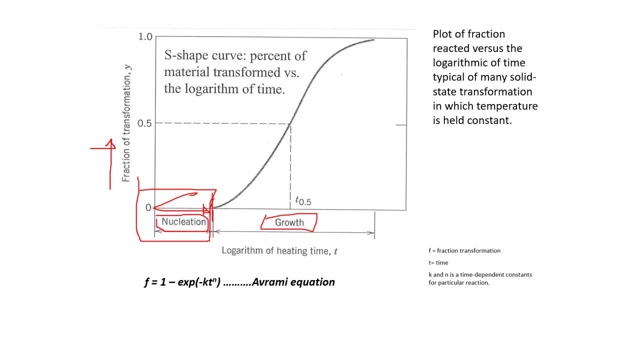 That's why The new, The new Product is different Due to the phase transformation Which, From It, is different from the parent phase. The transformation reaches the Completion If the growth of the new phase Over here The transformation. 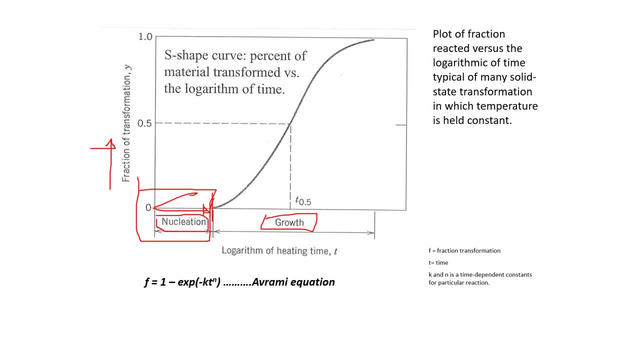 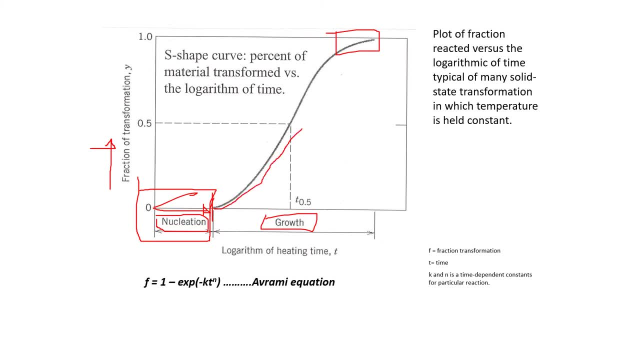 In the growth, or the growth increases exponentially, like over here in this, Until It Begins, It Comes to the stable Form. So This is the plot of friction: Reacted. What Is the logarithmic, Oliver? 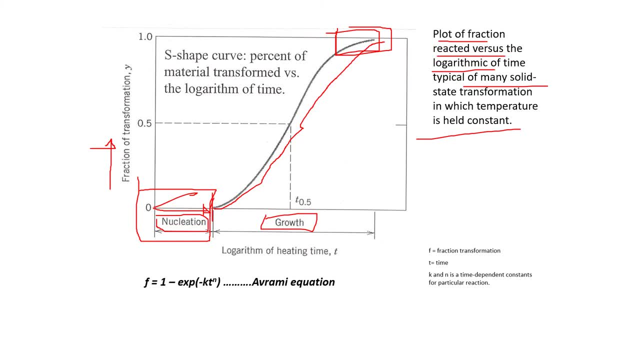 Display of time. Typically of many Solid Transformation in Western tonejis, Temperature, it's held constant. The s Shape Curve, the what. what is the logarithmic of time? this is the logarithmic of time. it shows the two types of. 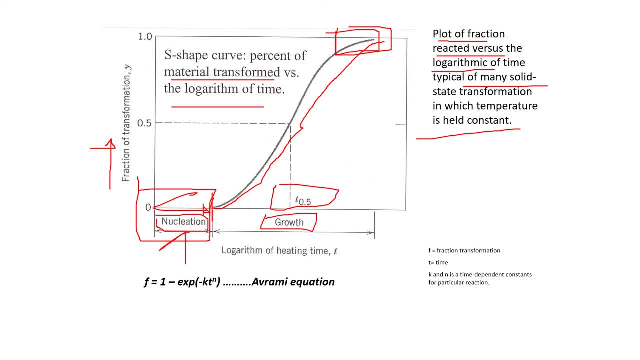 formation, phase, transformation: one is the nucleation, the other is group. the exponential equation is the our me equation. if is the friction, T is time, K and in other time dependent constants for particular reaction. so this is the equation in which are the s-type curve is formed. it is: 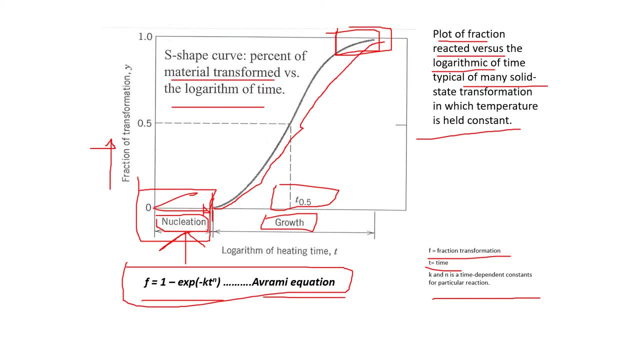 divided into two parts. one is the nucleation, the other is the group. first nucleation forms from starts from the few hundreds of atoms, and then the growth starts until it exponentially grows, until it reached the stables phase. in the stable phase the new constituent is different. 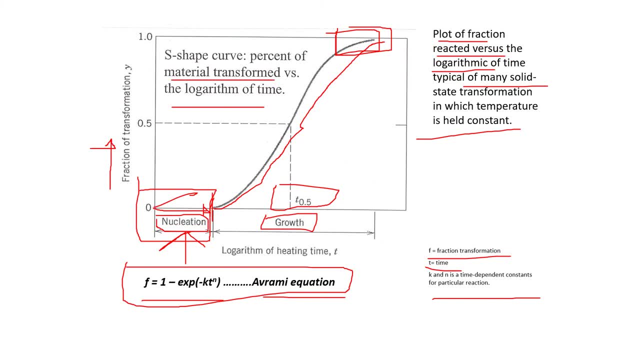 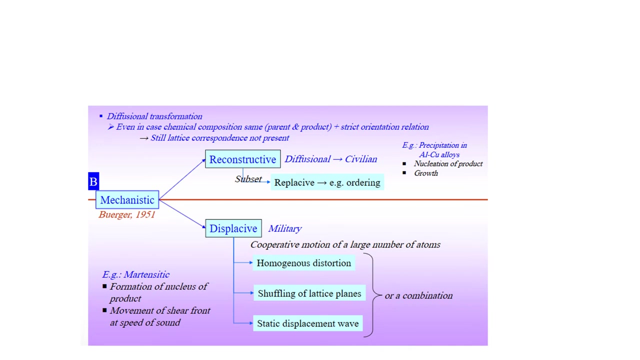 from the parent constituent and the new constituent is different from the parent phase. we the it is different from the parent phase. the transformation reached the completion over here in this stage and this point, the second type of for diffusion transformation is the mechanistic, which is further divided into: 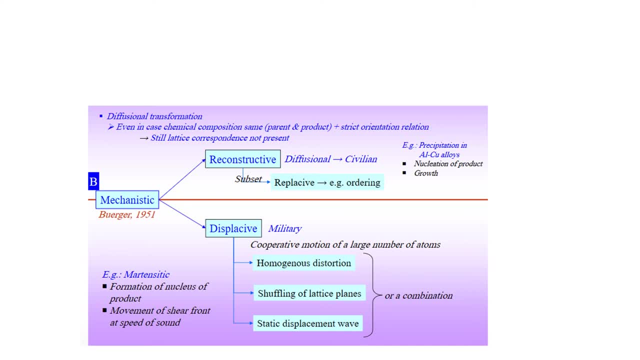 reconstructive. it has two parts: the constructive, different transformation, diffusion, transformation and display kill, transfer. reconstructive is a part of the constructive deformations- is sorry. reconstructive transformation is replicable and this is the display. the reconstructive deformation is civilian and they are. this piggy is military. 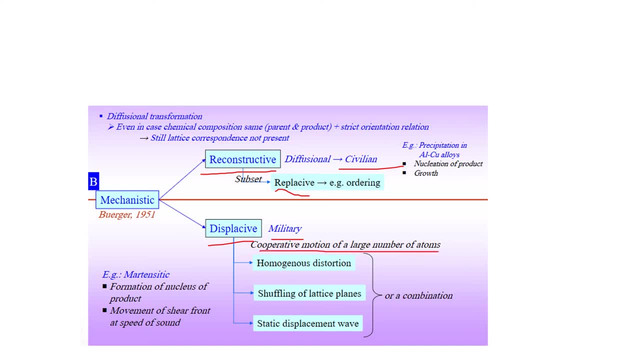 and over here in this idea. the example is a mud inside. formation of nucleus of products. movement of Eine. Video share for over here in display. you know the example is the modern site: formation of nucleus of product. One von heure over here in this picture: two returns as a contemporary. 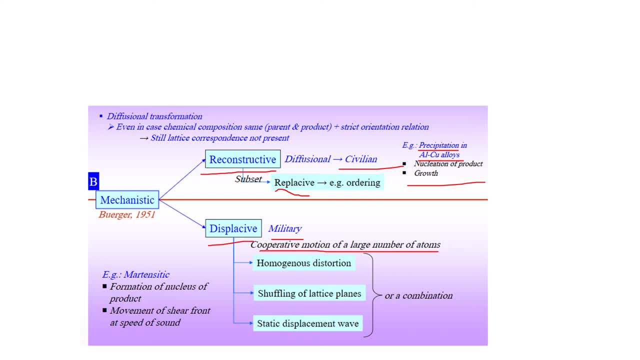 Ariana. Oh, so this is a presentation for the new based model of the old project, the producto, in recent negative- now I am going to- refined the wisdom between those movements of it so over of his mucus, their product, trying to return the size, and are satisfied to fill and move more a size. bigger pictures of the 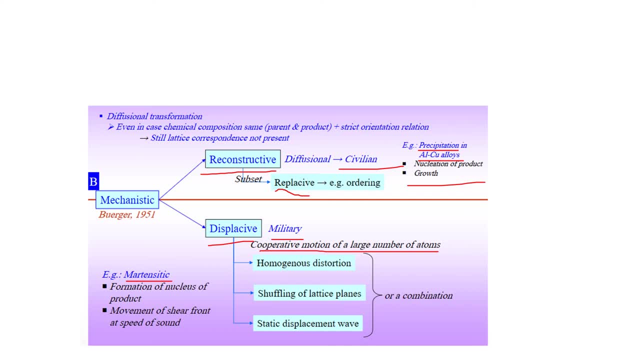 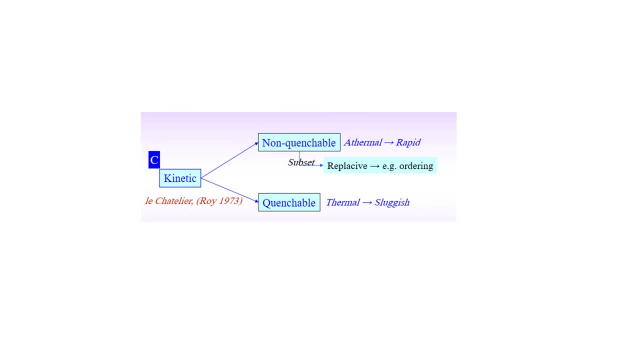 speed of sound. The third part for the diffusional transformation is kinetic. Kinetic can be further divided into quenchable and non quenchable, and quenchable. In quenchable, the process is athermal and rapid. In quenchable, the process is therma and sluggish. 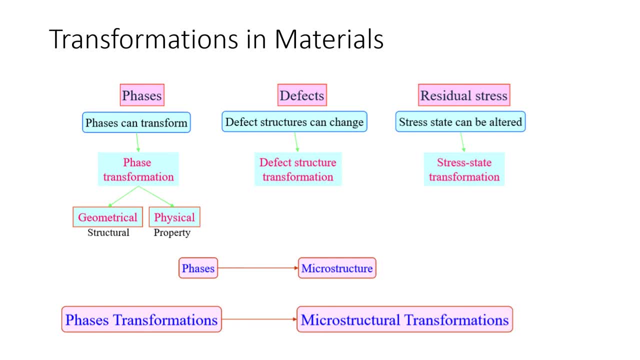 Transformation in materials. Here we further categorize the transformation of materials into three types. First one is we categorize into phases and then we study the defects of exhaust, And then we study the residual stresses either developed in the material while transformation, in the process of transformation. 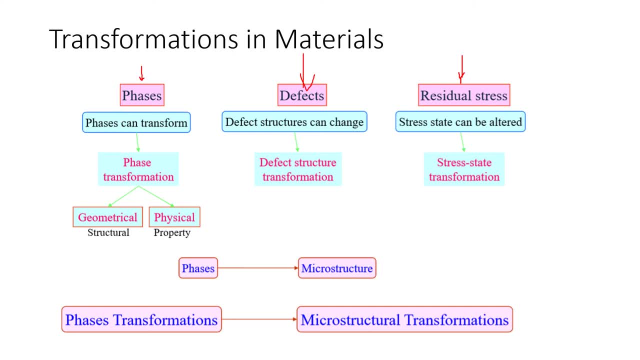 Phases can transform into geometrically or physically. The geometrically we discuss the structural behavior and physically we discuss the property Defects. we have already studied about the defects, like voids, like the microstructure transformation. Defect structure can change, defect structure can change the defect structure transformation. 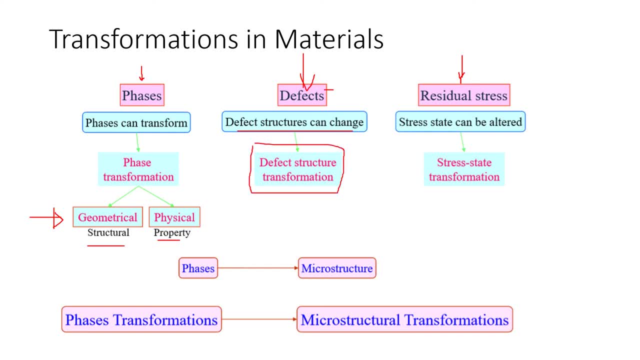 During the formation of, During the formation of, During the phase transformation. some defects can also be found out during the phase transformation. The residual stresses. some residual stresses are developed in the structure during the phase transformation, like stress state transformation. So for the phases: 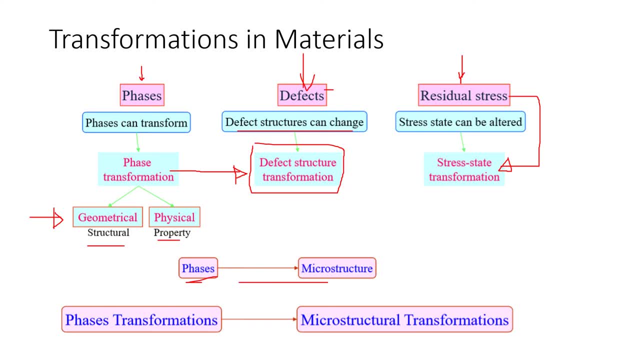 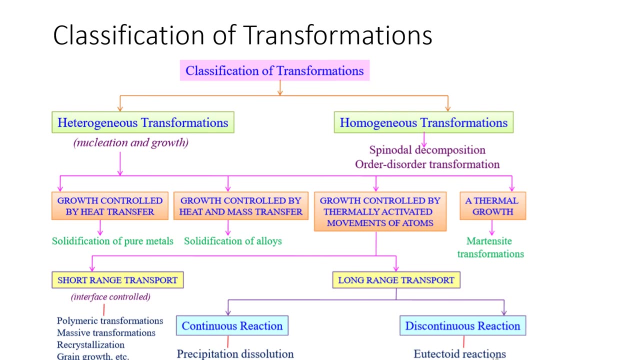 We study the microstructure Phase. transformation is actually subjected to microstructure transformations. We can further classify the transformations. Classifications of transformation can be further divided into two types of homogeneous and heterogeneous transformation. Homogeneous transformation- Transformation- Homogeneous transformation is actually a homogeneous transformation. 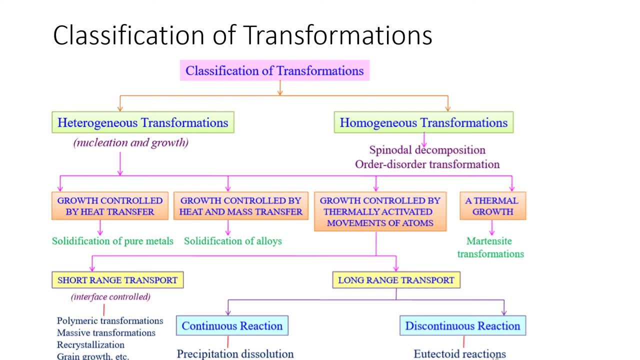 Nuclei form uniformly throughout the parent phase. It requires considerable super cooling between 80 degrees centigrade to 300 degrees centigrade Homogeneous nucleation- So in homogeneous nucleation- is actually categorized For the temperature range. formation of temperature range. 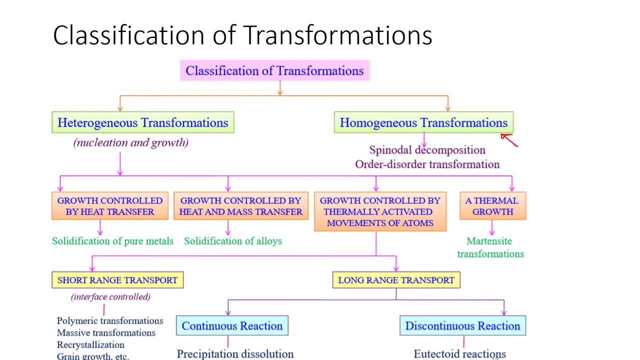 The heterogeneous. homogeneous needs super cooling, While heterogeneous form a structure in homogeneities Like container surfaces, impurities, grain boundaries, dislocations and liquid features, Which is much easier since stable nucleation surface. It is already present. 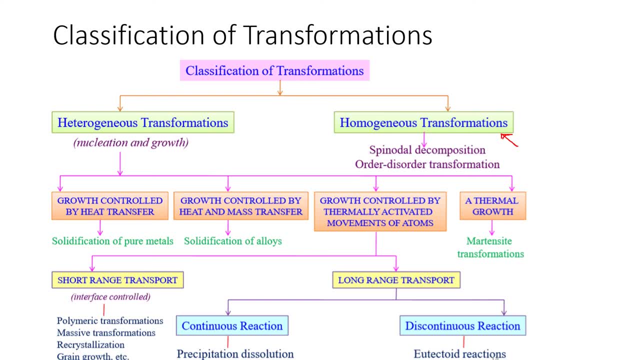 It requires slight super cooling Which is between 0.1 to 10 degrees centigrade, Mainly if we want to memorize between the classification of homogeneous and heterogeneous. Homogeneous requires super cooling Which is at the range of between 800 to 300 degrees centigrade. 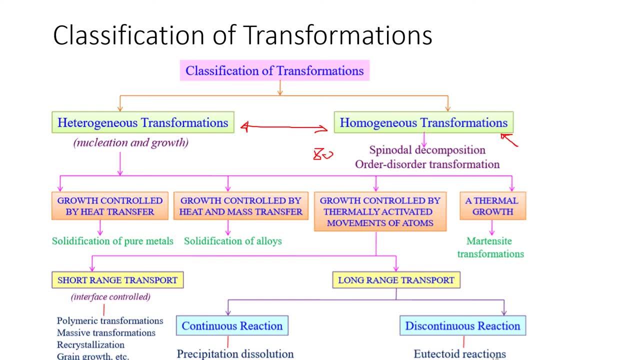 Starting from 800 to 300 degrees centigrade, While heterogeneous transformation- For the heterogeneous transformation, The temperature range is slight. super cooling, Which is between 0.1 to 10 degrees centigrade. The examples are the inhomogeneities. 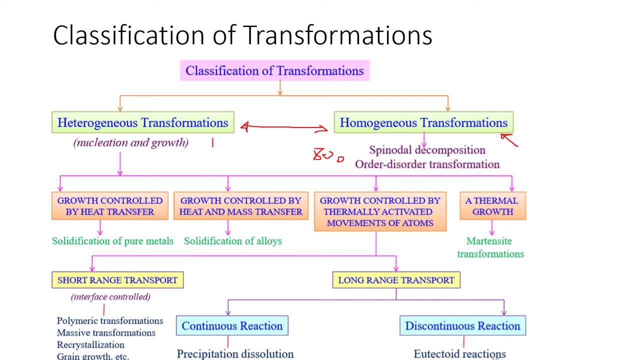 Like container surfaces, impurities, grain boundaries and dislocations In heterogeneous, homogeneous transformation. we already we also studied the nucleation and growth. The nucleation and growth can further be divided into the following categories. In these categories, the growth controlled by heat transfer, growth controlled by heat and mass transfer. 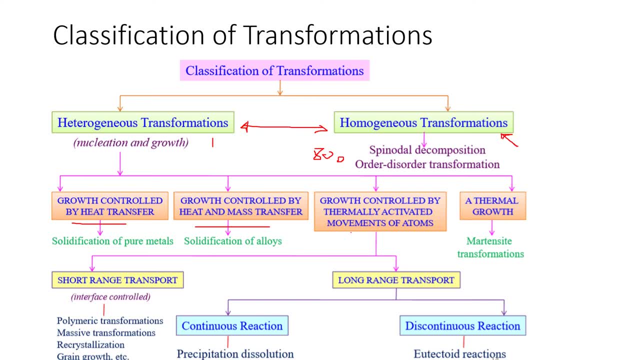 growth controlled by the thermally activated movements of atoms. thermal growth, which is a thermal growth which is the example, is martensite transformation In growth controlled by heat transformation. the process is solidification of pure metals In growth controlled by heat and mass transfer. 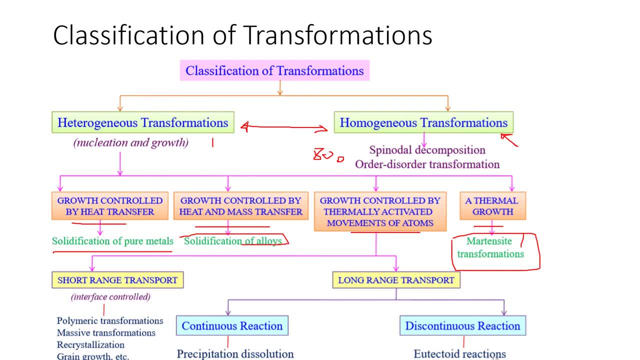 the growth is followed by the solidification of pure metals, The solidification of alloys, solidification of alloys. Further, if we want to differentiate between the growth controlled by heat transfer and growth controlled by heat and mass transfer By heat transfer, actually we studied for the pure materials. 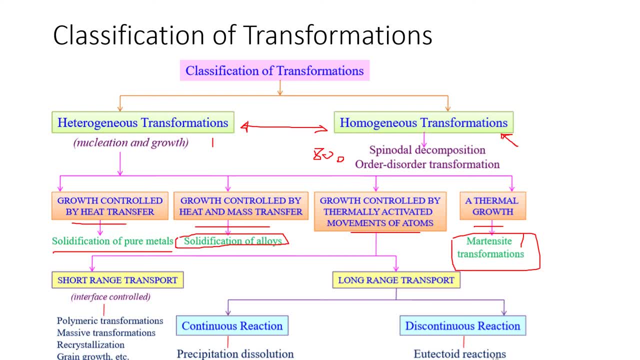 By heat and mass transfer. we study the alloys. solidification of alloys. Growth controlled by thermally activated movements of atoms are categorized into two types: Short-range transport and long-range transport. The short-range transport is actually meta. is the interface controlled. 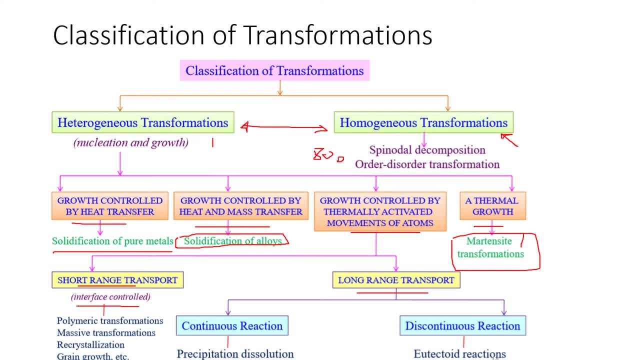 It is actually metastable and interface controlled. It is polymeric transformations. The types are for the short-range transport. the examples are the polymeric transformations, massive transformation, recrystallization and growth grain growth, While the long-range transport can be further divided into two categories. 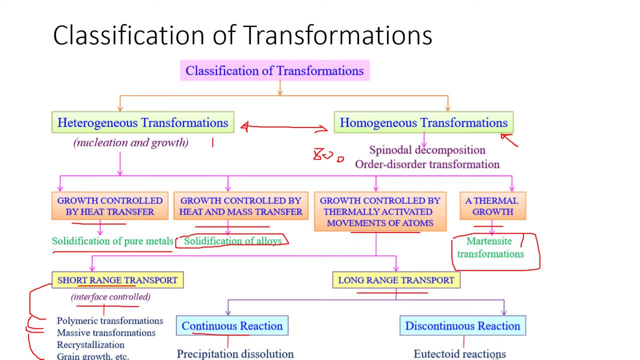 One is the continuous reaction, the other is the discontinuous reaction. In continuous reaction the precipitation dislocation occurs. One of the example of the discontinuous reaction is the eutectoid reactions. This is the classification of transformation. In exam you may be asked to summarize the classification of transformation. 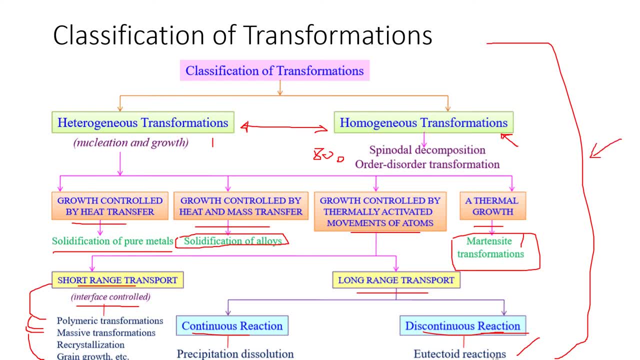 which is given in this flow chart. Actually, in this flow chart, first you will divide the classification of transformation into two categories: homogeneous and heterogeneous, And then you will explain what is homogeneous transformation, what is the heterogeneous transformation You can only study about. you can give the examples of homogeneous transformation. 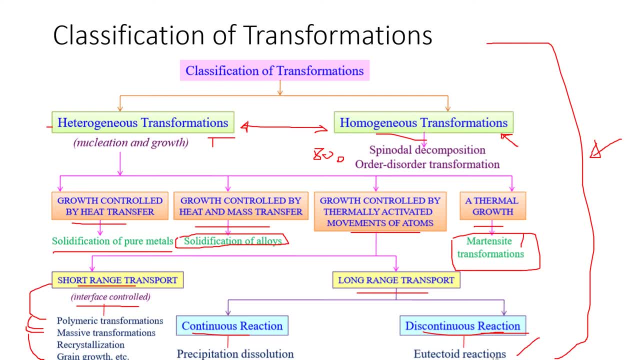 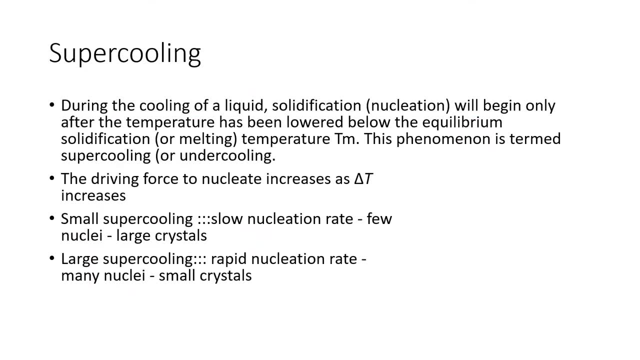 and heterogeneous transformation. Further we will explain some basic reactions and equations We have. while explaining the classification of materials and classification of transformation, we have discussed about the super cooling. Now we further explain the super cooling During the cooling. it is one of the process of the homogeneous and heterogeneous transformation. 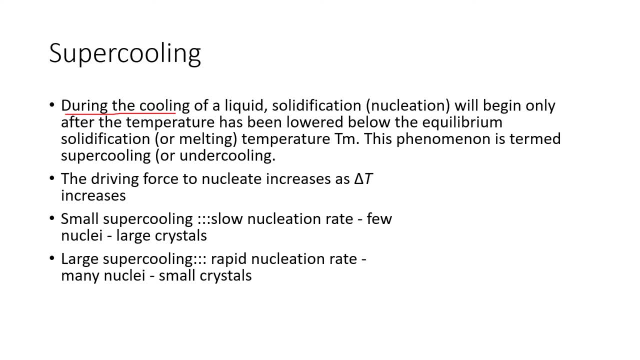 During the cooling of a liquid. solidification or nucleation will begin only after the temperature has been lowered below the equilibrium solidification or melting temperature, as we have discussed in the eutectoid formation. In eutectoid formation, we have discussed about the eutectoid temperature. 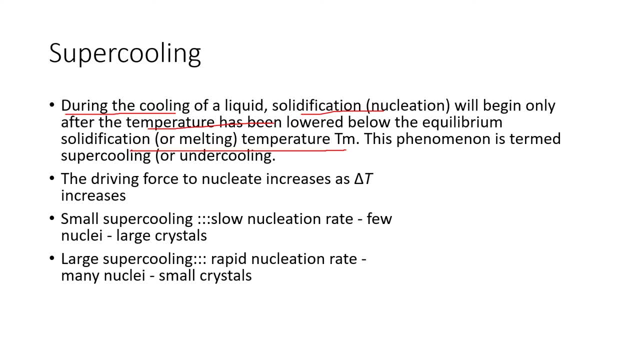 Once it is below the thermal temperature, or thermal equilibrium, or over. here we discussed below the equilibrium solidification. Both have the same meaning. This phenomena is termed as super cooling or under cooling. The driving force to nucleate increases, the delta T increase. 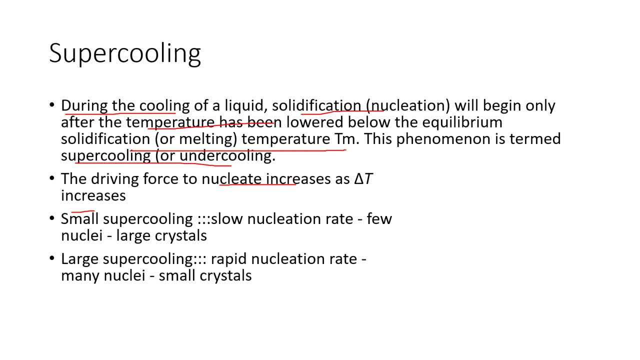 The driving force increases. What is the driving force? What is the behavior of the driving force? or what is the action of the driving force? This driving force is used to nucleate. This increase is the delta T increase For the small super cooling slow nucleation rate. 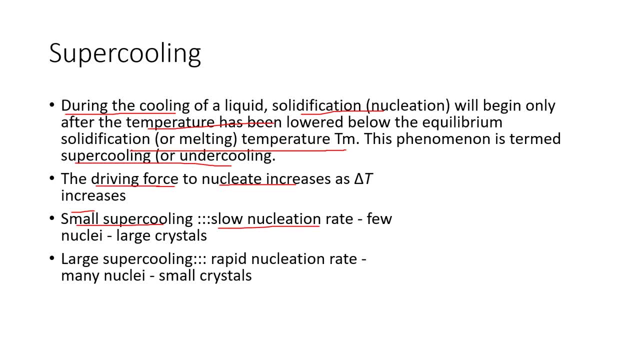 the nucleation rate is slow and few nuclei are formed, but large crystals are formed. For large super cooling it is a rapid nucleation rate and many nuclei forms, but the crystal formation is small. We can differentiate between the small and large super cooling. 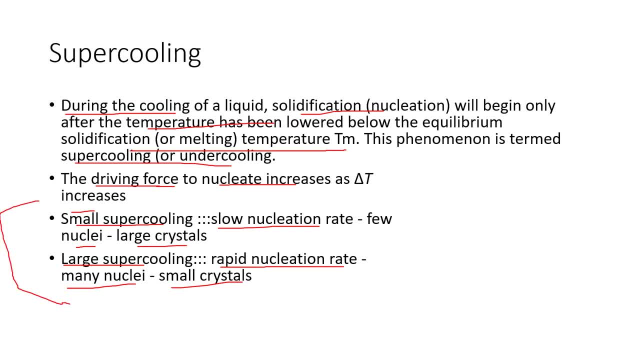 For small and large super cooling. for small super cooling few nuclei are formed, the nucleation rate is slow, While for large super cooling nucleation rate is rapid and many nucleations are formed, but the crystal formation is small, While for small super cooling crystal formation is large. 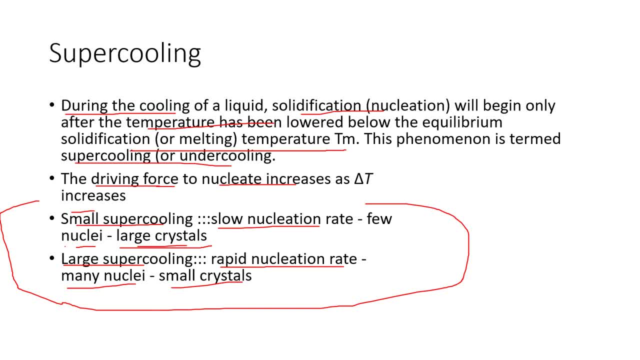 This is the main difference between the small super cooling and large super cooling. We have discussed in classification of transformations that the temperature range for the homogeneous and heterogeneous transformations, For one transformation we give the heat between 800 to 300 degrees centigrade. 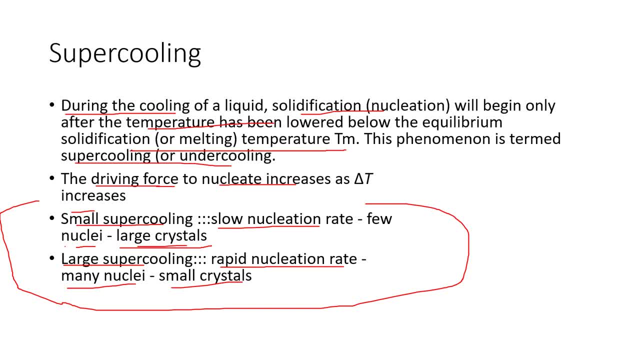 while for the other type of transformation we give the temperature. The temperature range is between 0.1 to 10 degrees centigrade only. This depends upon the formation of small crystals and large crystals. Now we will discuss about the nucleation and growth mechanism. 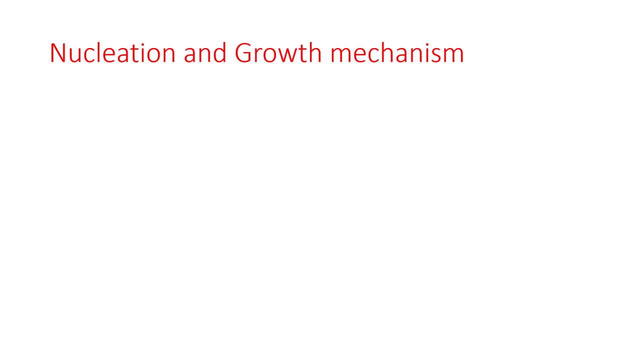 We will discuss this in detail in the upcoming lecture. However, in this lecture we will define a short summary of the nucleation and growth mechanism, just like we have discussed in exponential growth and nucleation In the nucleation stage. nucleation starts only from few hundred of atoms. 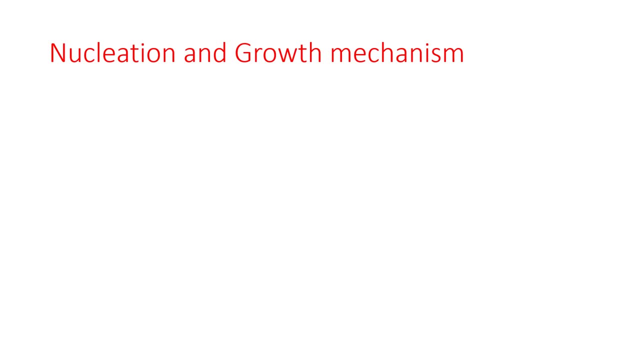 From the beginning of the transformation, of phase transformation, while once the nucleation forms, after that only few crystals are formed. After that the growth starts: Growth of that crystal, growth of the nucleus begins to form. The growth mechanism is discussed by one exponential equation. 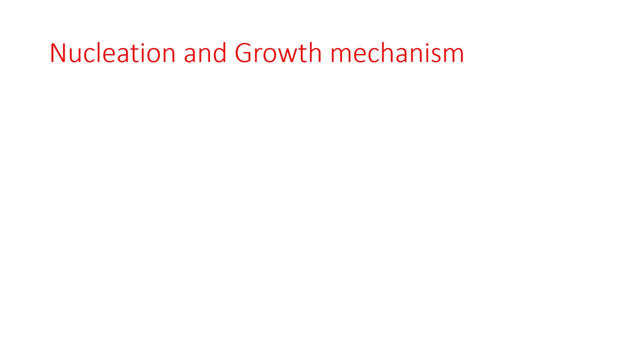 that we have already discussed in S-type of curve, In that exponential equation it starts exponentially, The growth starts exponentially And once it reaches a stable phase, the end of the S portion, then the solution, the new constituent, the new form.